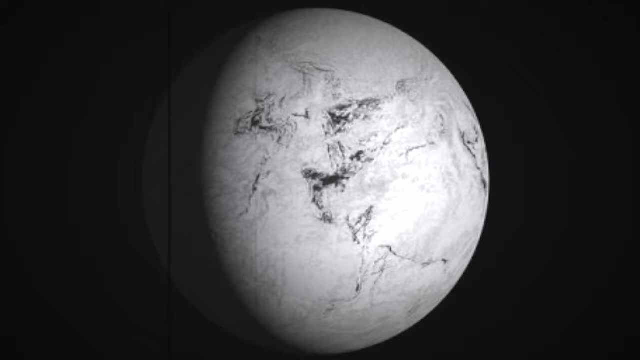 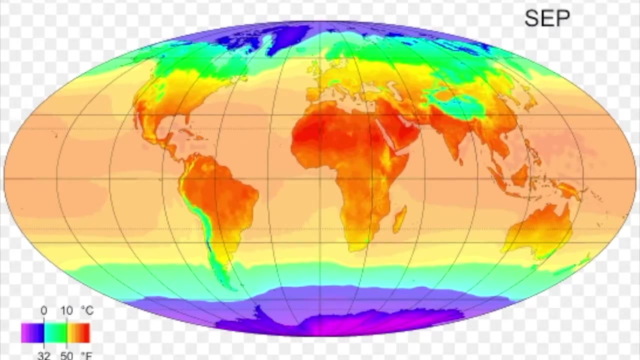 More specifically, it helps us find out what our Earth's climate was like before we started keeping the meticulous direct climate records which give us a very accurate view of what our climate is like today. So now that you know what paleoclimatology is, you may be. 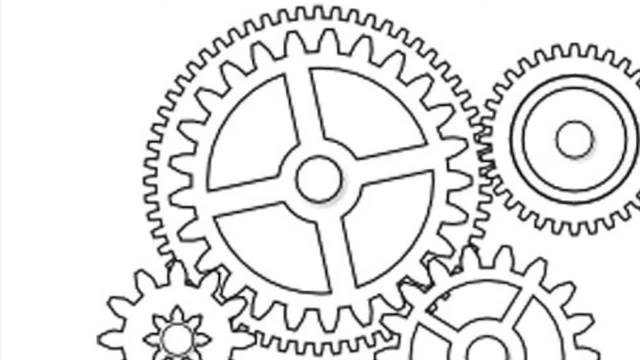 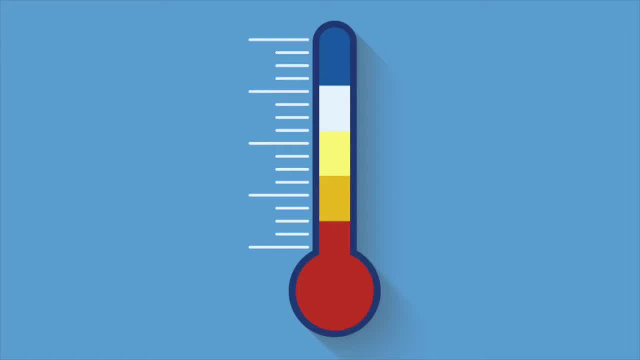 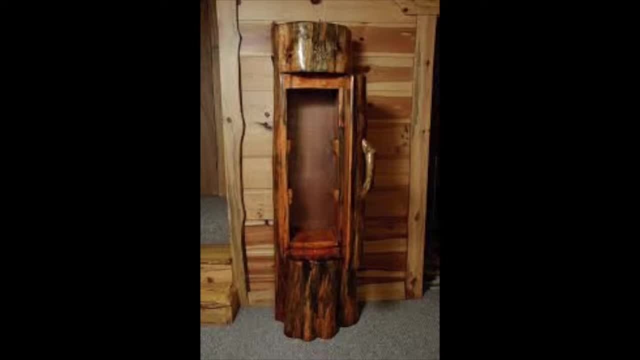 wondering how does it work? Paleoclimatologists use what are called proxy records to gain quantitative data on various measures relevant to climate, including temperature, rainfall and the concentration of certain gases. Proxy records are natural archives which store climate information through a variety of methods which differentiates them from direct records. 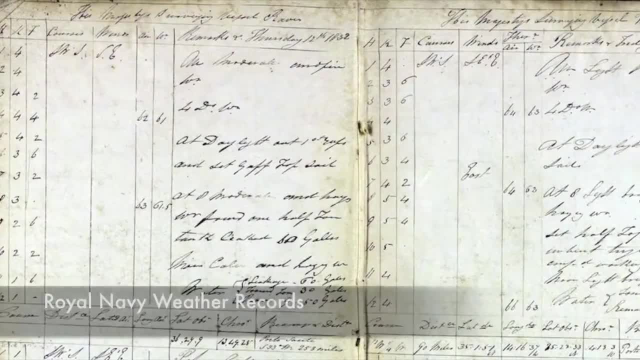 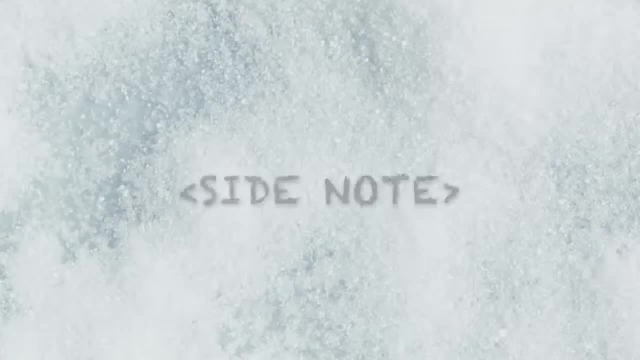 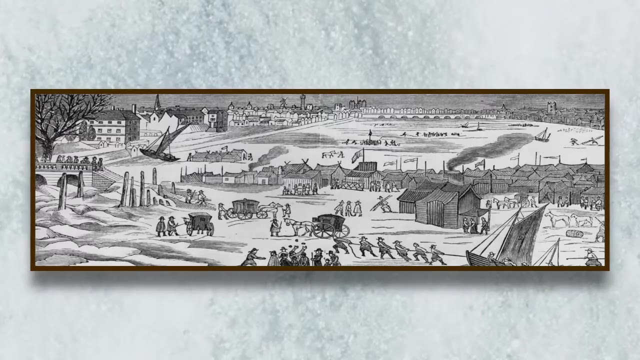 as those are made by us humans: Proxy record- direct record. proxy record- direct record- proxy record- direct record. While paintings are human made, they do not directly provide us with quantitative climate data and are therefore indirect proxy records. Direct records must be human made and directly. 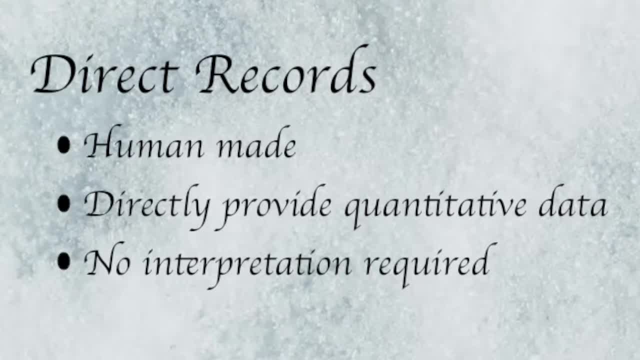 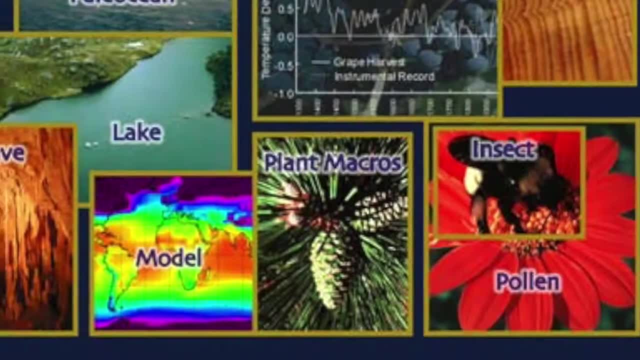 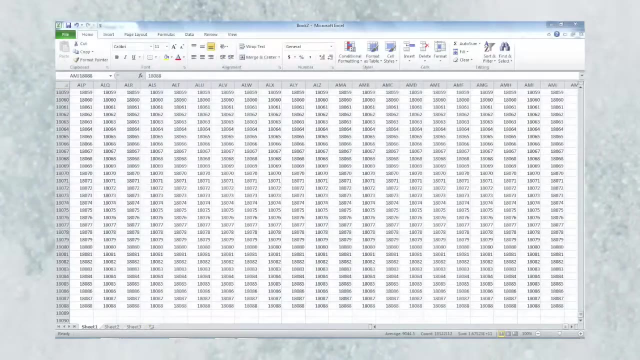 provide us with quantitative data with no interpretation required. Each proxy record is different, with different information stored, different methods of storing this information, different degrees of accuracy and various start times. But when these records are compared with direct records and each other, and if the sample size is large enough, they can. 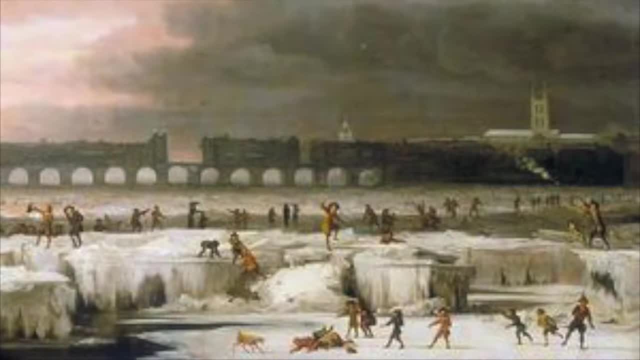 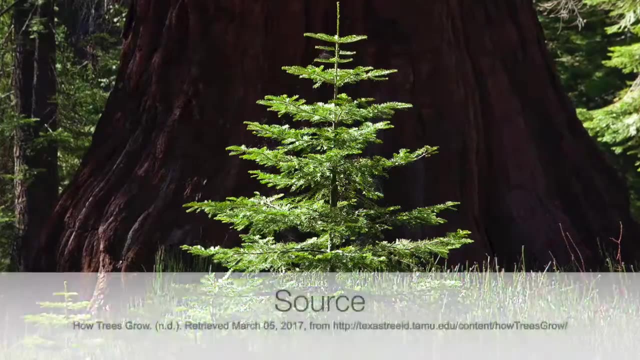 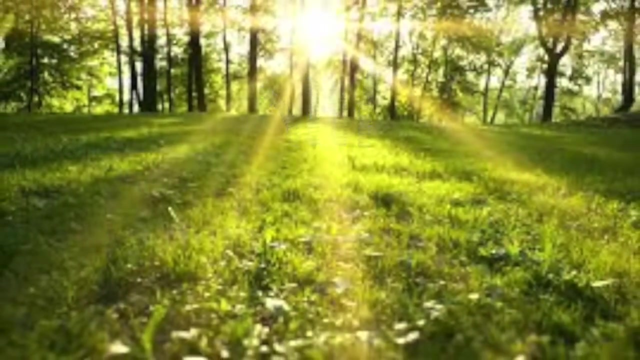 give us a fairly accurate picture of what our climate was like at different points in the past. As trees grow, they go through two growth cycles per year, During the spring and early summer. the tree does most of its growing due to the wetter conditions at this time. 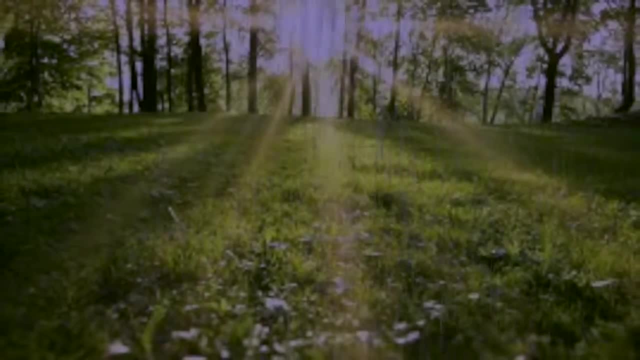 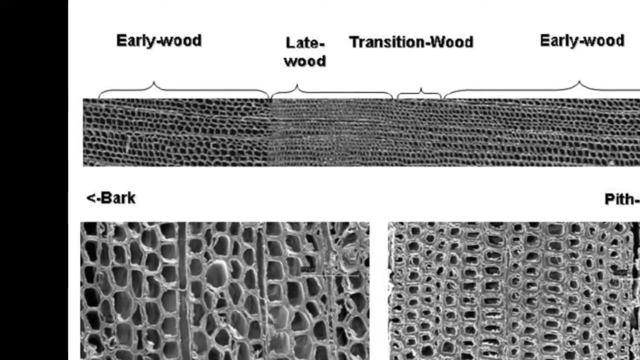 of year. During this cycle, the tree grows large cells with thin cell walls, producing a lighter colored wood, known as the early wood. In the late summer and the fall, the tree begins to produce wood at a slower rate and the cells produced are smaller and have thicker 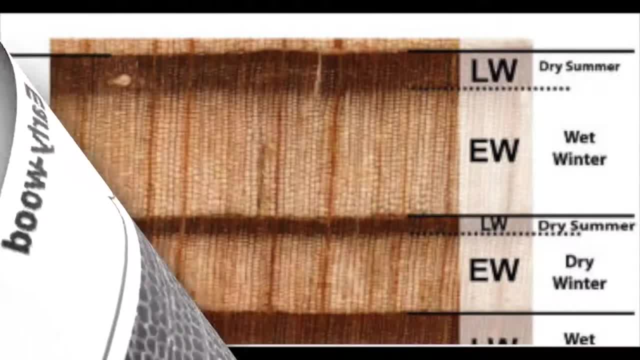 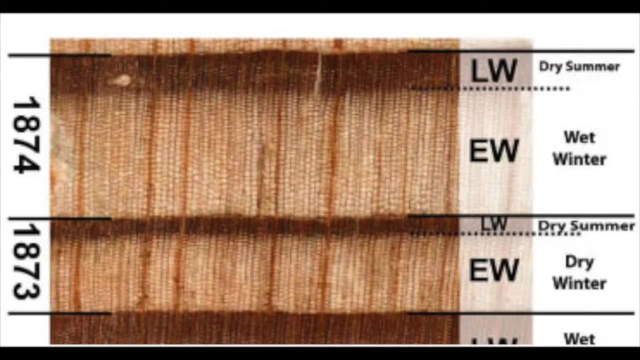 cell walls, creating darker colored wood, known as the late wood. The cycle repeats itself every year and the thickness of both the light and the dark rings indicate how favorable the climactic conditions of that year were to that tree's growth. The thicker the rings, 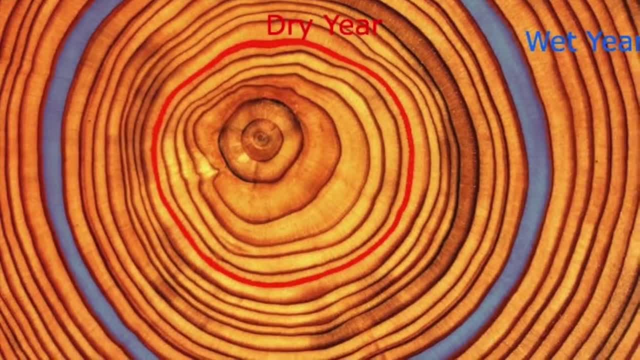 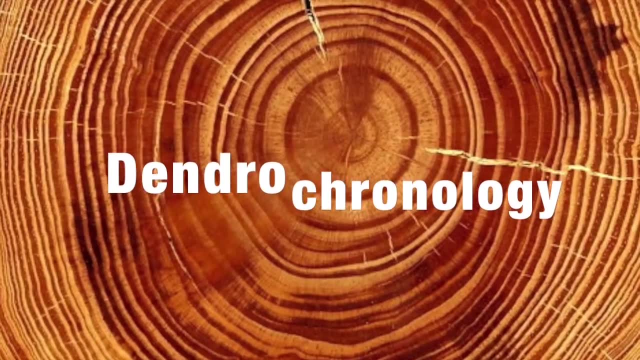 the more favorable growth is. The more favorable growth is, the more favorable growth is. The growth process is an integral part of Dendrochronology. Dendrochronology, or tree dating, is the science of determining what our climate was like in. 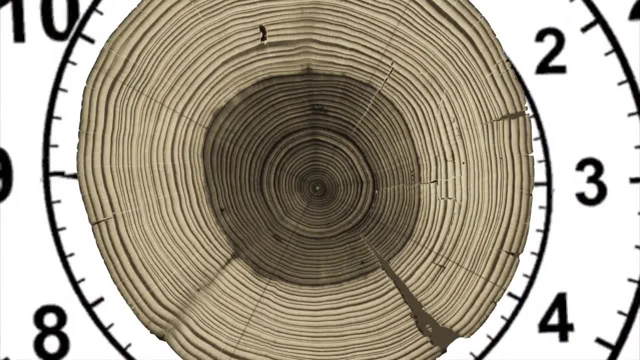 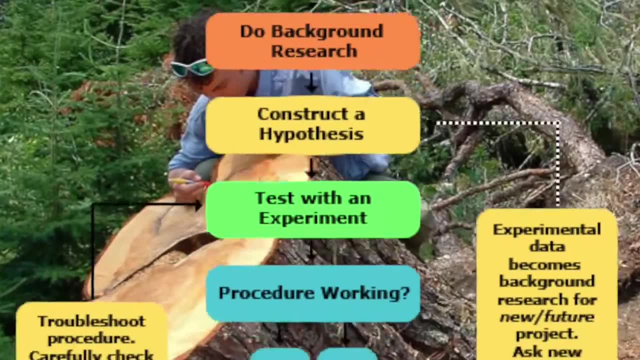 the past, using the annual growth rings on trees. based on the principles mentioned earlier, Dendrochronology, like all other good science, is conducted in accordance with the scientific method. Dendrochronology starts off by asking a question similar to the question of the tree called. 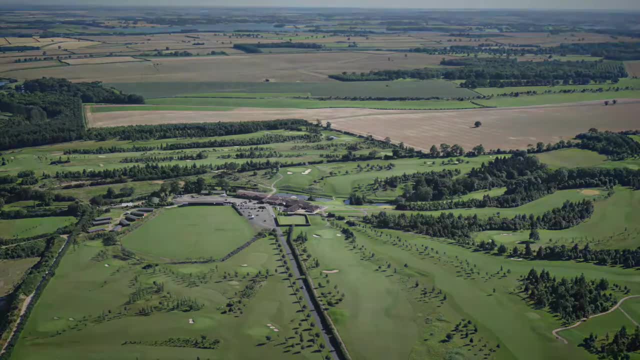 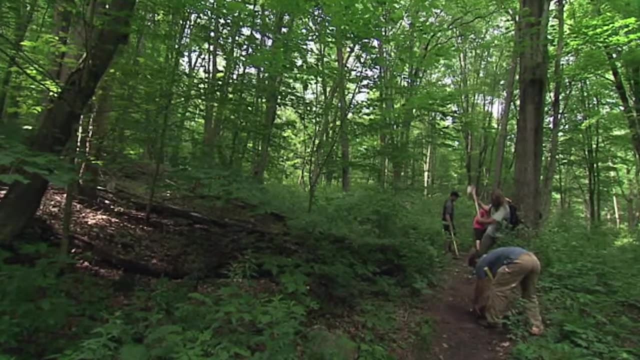 to what was the climate of insert area here, like in the past. They then form a hypothesis based on both direct records and indirect proxy records for that area. After that they conduct their experiment and take samples from a large number of trees. 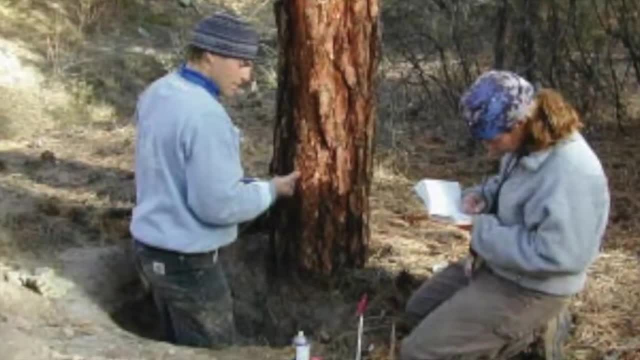 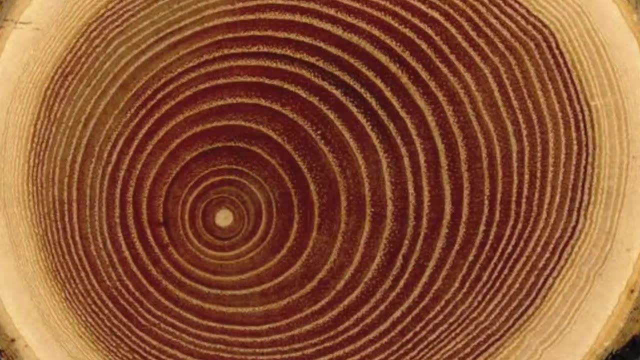 in an area, Dendrochromologists take two types of samples: cross-sections and increment cores. Cross-sections are better than increment cores as they provide a full view of all the rings, allowing any irregularities to be taken into account. 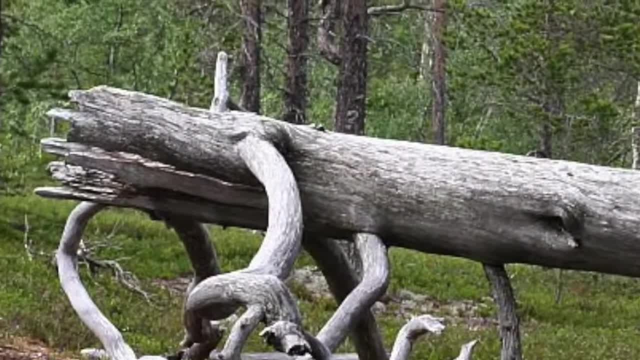 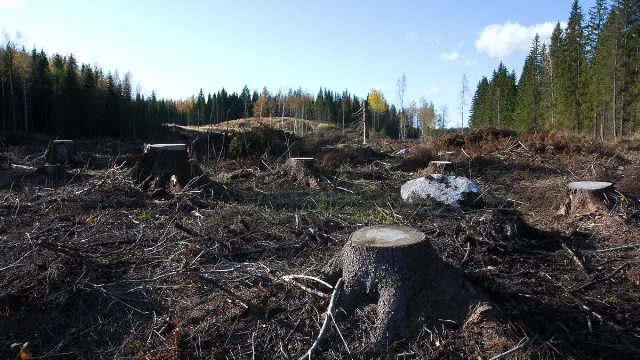 But cross-sections can only be taken from dead trees, as taking a cross-section from a live tree would most certainly kill it And, due to the large sample size needed to ensure accurate results, a large chunk of the forest would be leveled by the end of the experiment. 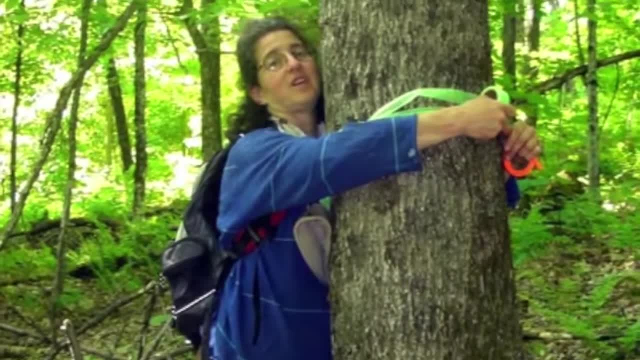 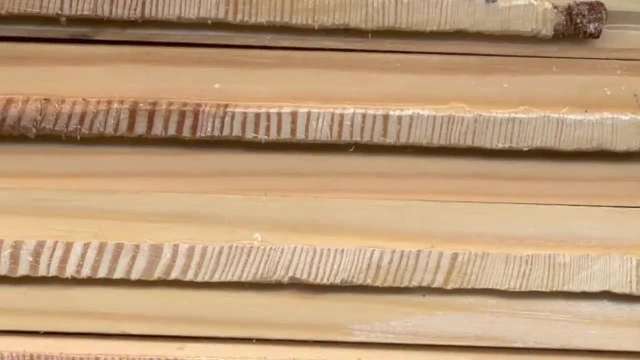 To avoid this problem and the wrath of hippies everywhere, dendrochromologists use increment borers to drill long, narrow increment cores out of the trees. This does not kill the tree, as it only takes away a small amount of wood To avoid any irregularities. 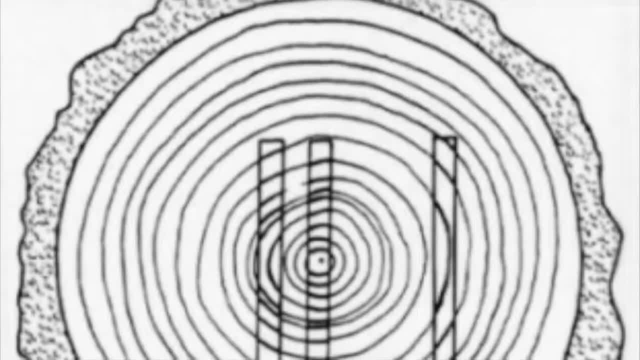 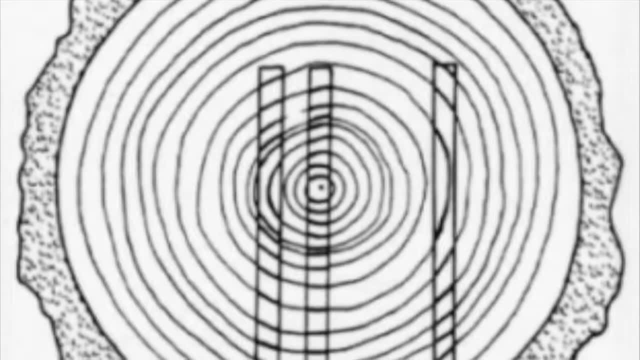 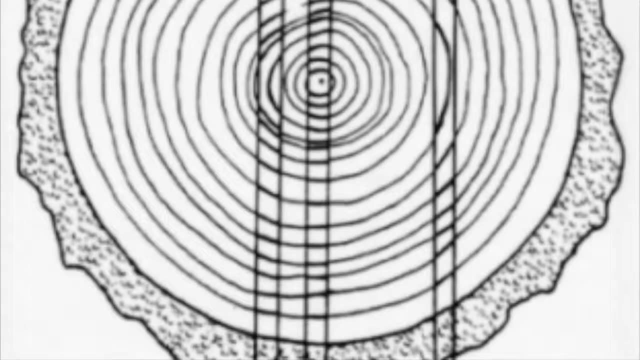 being misinterpreted as tree rings. dendrochromologists often take multiple cores from a single tree at various heights to ensure the most accurate results possible. Side note: when you are taking increment cores, it is essential that you include the pith or center of the tree in your increment core, or else you will be unable to date the sample. 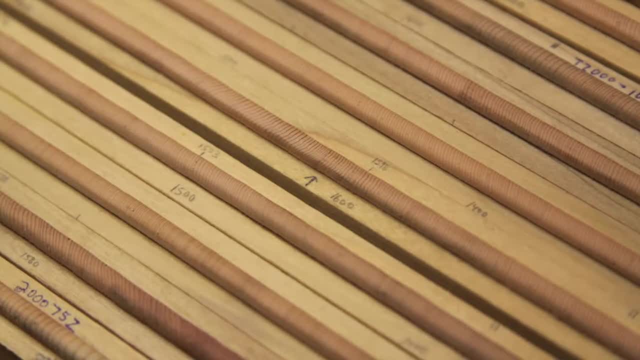 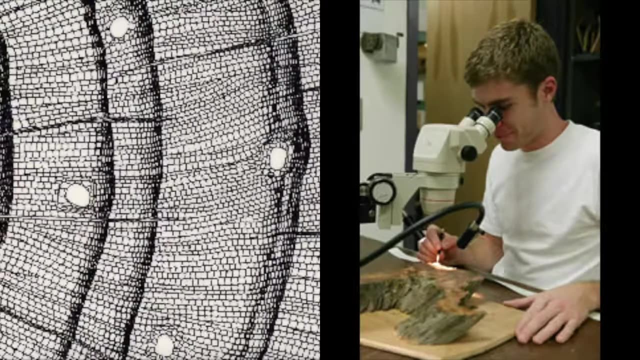 In this case, cores A and C are useless. After dendrochromologists take a large number of samples from an area. the samples are observed under a microscope. Dendrochromologists count the tree rings and determine how old the tree was when it. 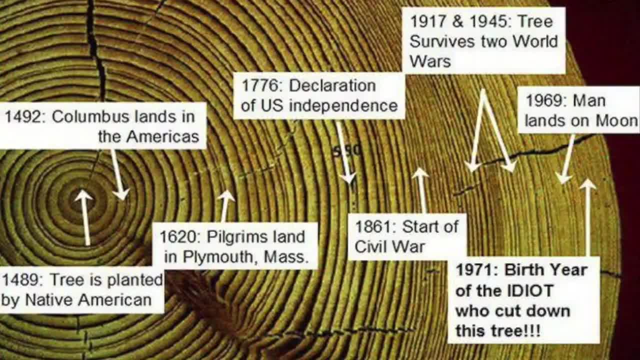 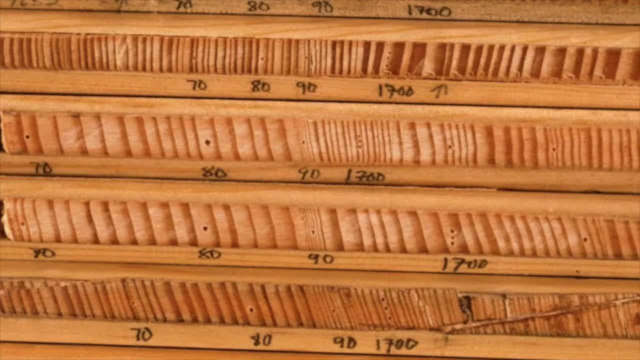 began growing. so they can associate each of the growth rings with a year. For cores taken from living samples, this is done by marking the last complete growth ring and associating it with the year before the sample was taken. The rings are then counted from outermost to innermost, determining which year each ring. 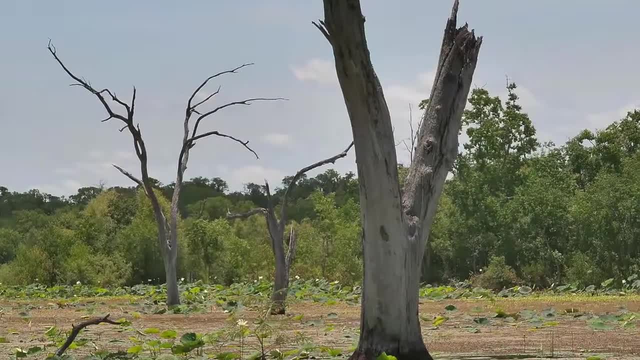 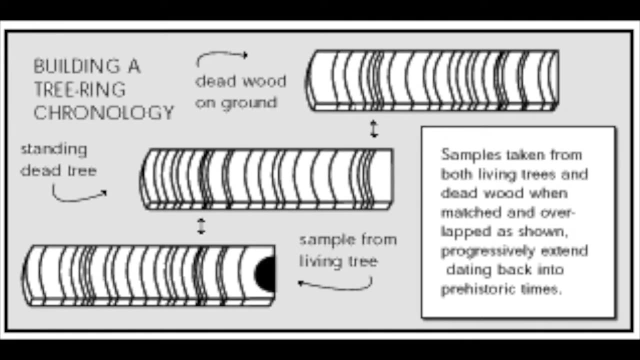 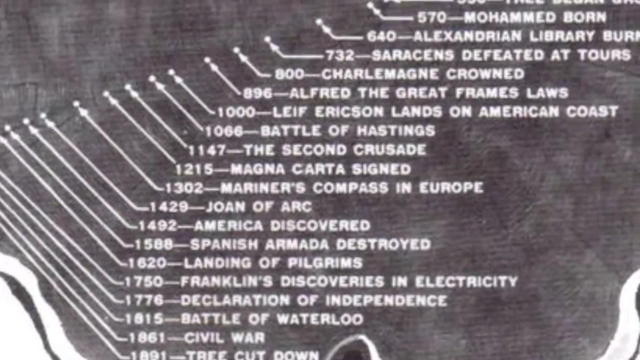 was from. For cross sections taken from dead samples, they must first be cross-dated with living samples from the same area and preferably of the same species species to determine which year the uttermost complete growth ring is from. After this has been done, each growth ring is associated with a year, using the same 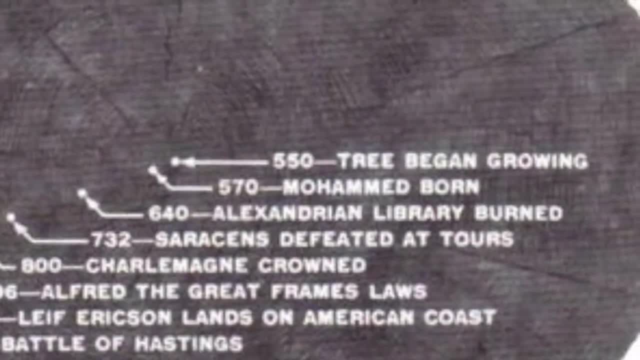 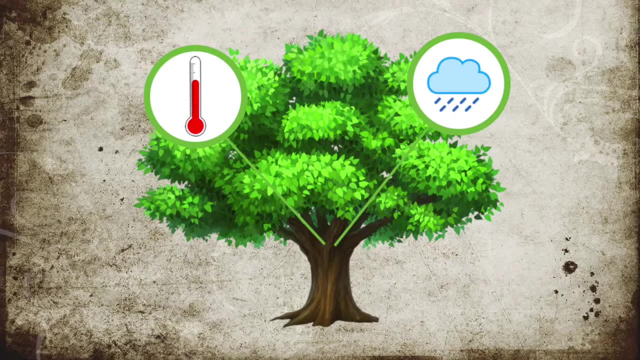 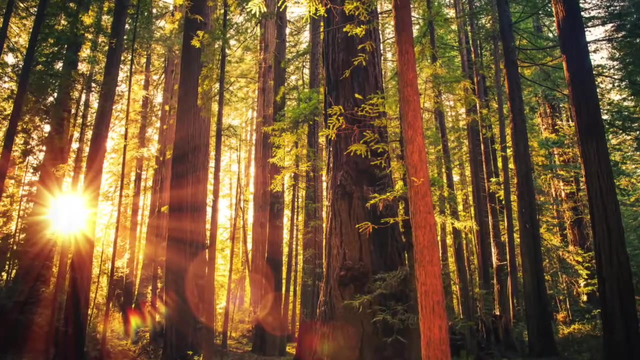 method as the living cores. After the rings have been dated, the preferred growing conditions of the species of tree the sample came from are taken into account, so scientists can compare the characteristics of the tree rings to certain climactic conditions, For example, the California Redwood, a favorite of dendrochromologists due to its long lifespan. 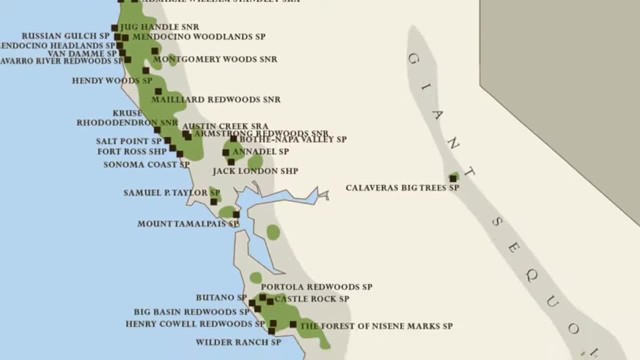 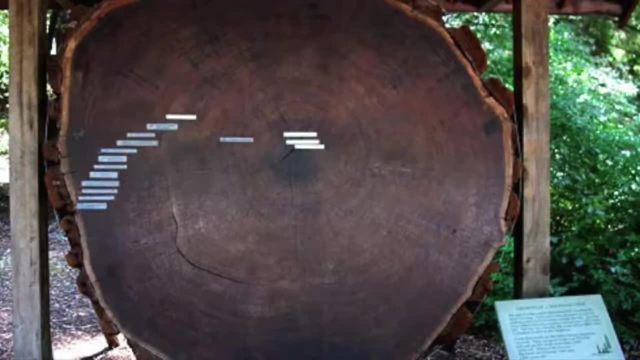 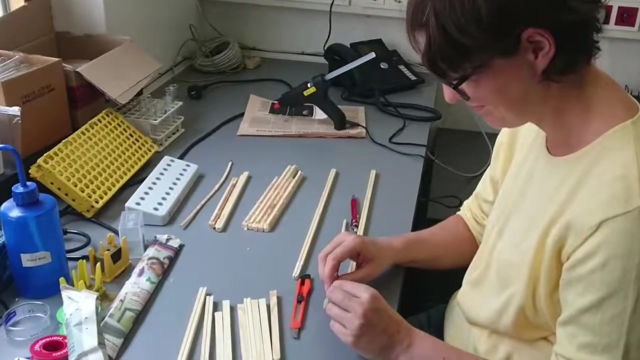 and resistance to rotting refers oceanic climates with high amounts of humidity, fog and therefore moisture, and relatively low temperature variation. The years with the widest rings can be associated with years where these conditions were most prevalent. After all, the rings have been interpreted. samples are compared with each other previously. 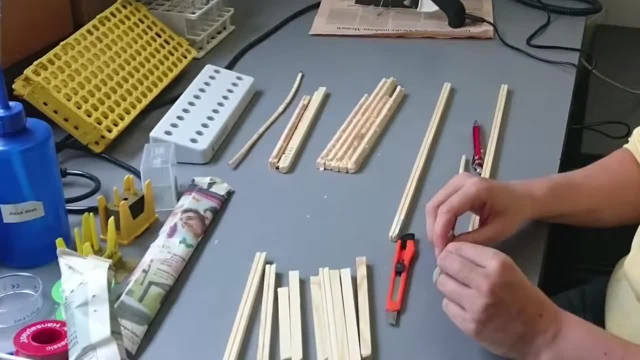 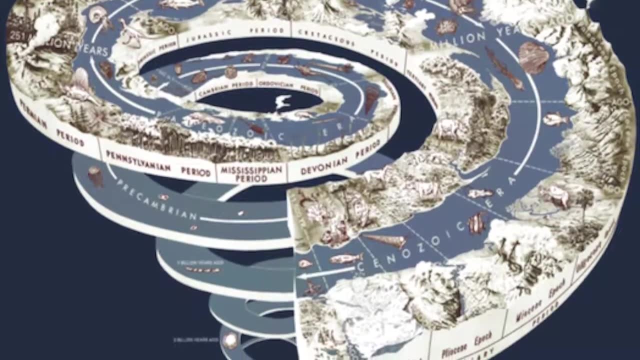 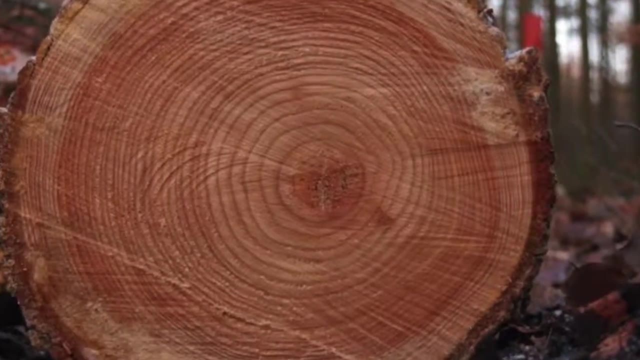 taken samples, other proxy records and direct records for the area. Based on this data, dendrochromologists then come to a conclusion as to what the climate was like in the past for a certain area. There are a couple of problems with using trees as a proxy record. 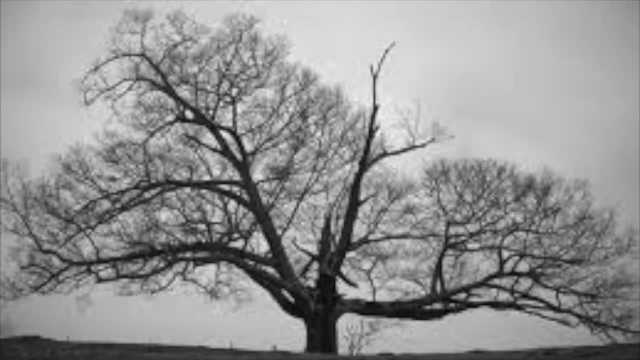 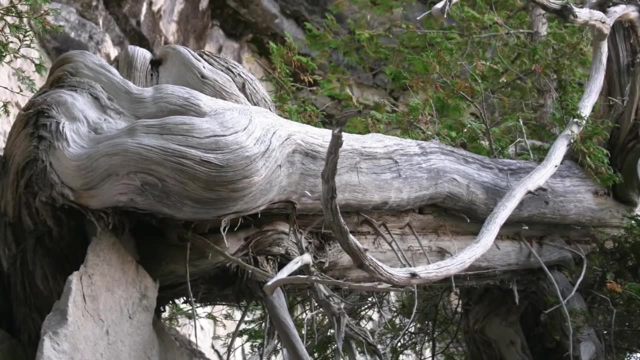 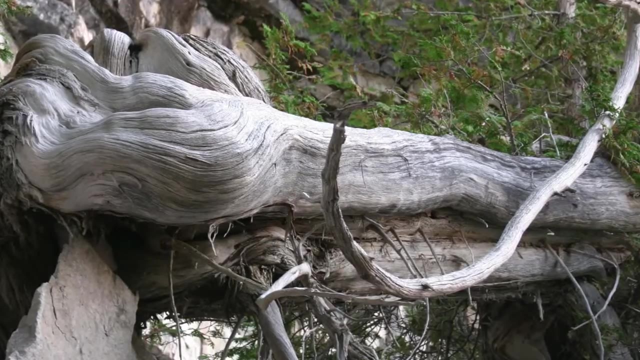 The first problem is that trees can only live so long, so the records only date back to the birth date of the oldest sample we can find. This can still carry us a long way into the past, with trees like the Eastern White Cedar found on the Niagara Escarpment of Ontario dating back up to 2,767 years, and the Hohenheim. 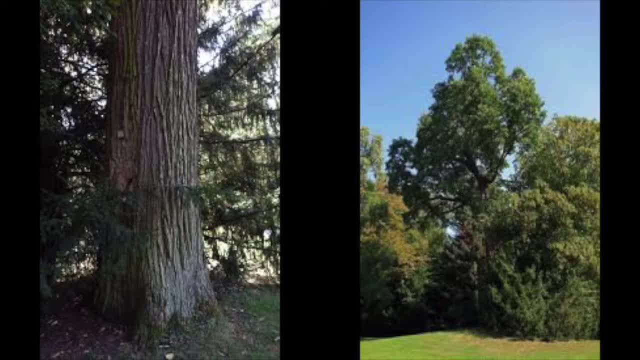 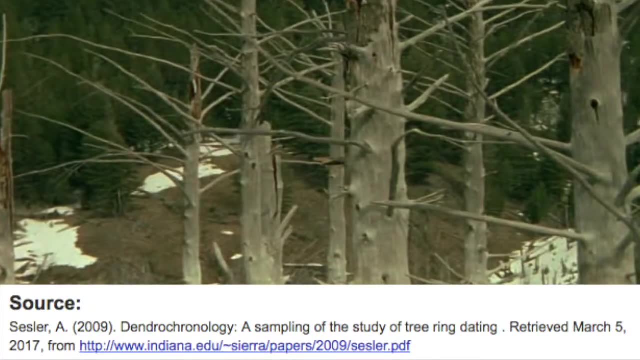 Oak found in Germany. This has given us climate records dating back 12,500 years. Furthermore, dead tree samples that have been preserved in ice or other mediums can be cross-examined with living samples, giving us records that date back even further. 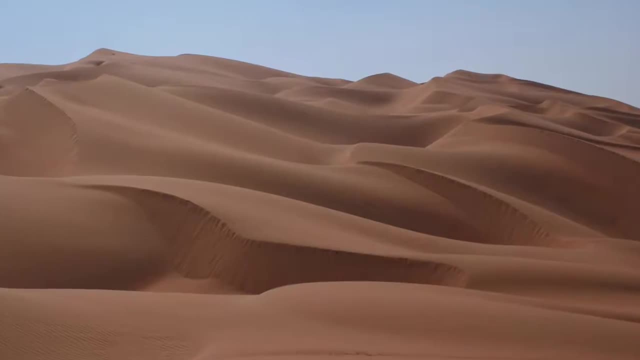 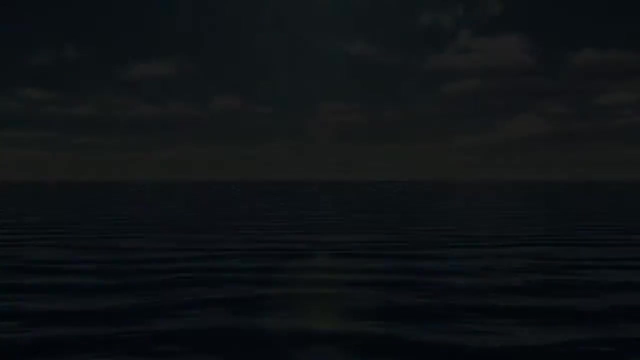 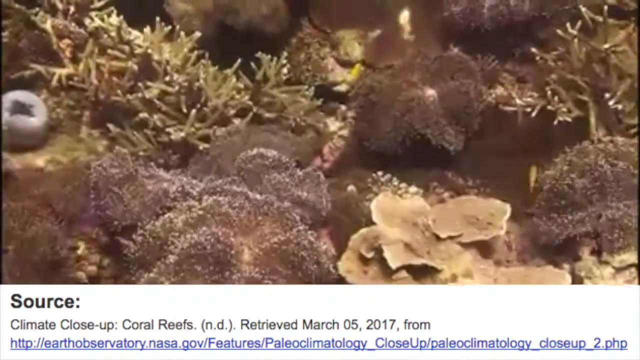 The second problem is that trees do not grow everywhere. Areas like deserts, the Arctic and our oceans do not have trees growing in them, So how do we get climate records from these areas? When it comes to paleoclimatology, coral reefs are the forests of the ocean. 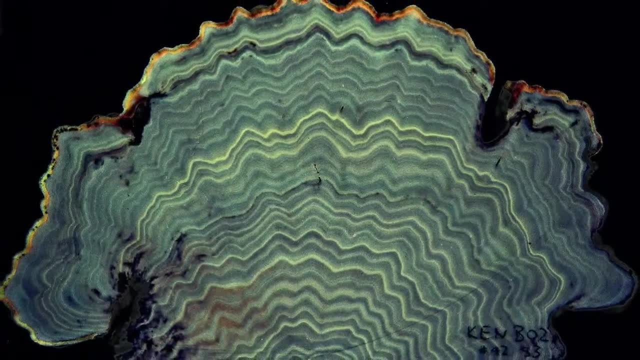 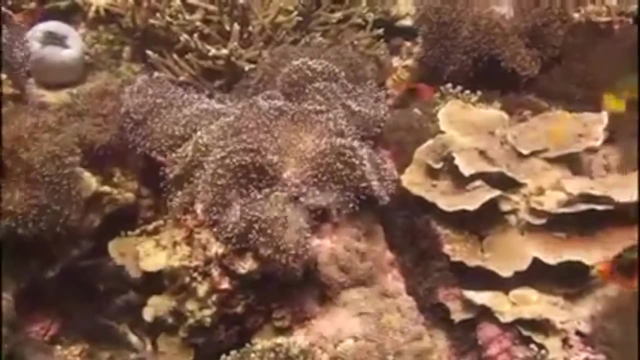 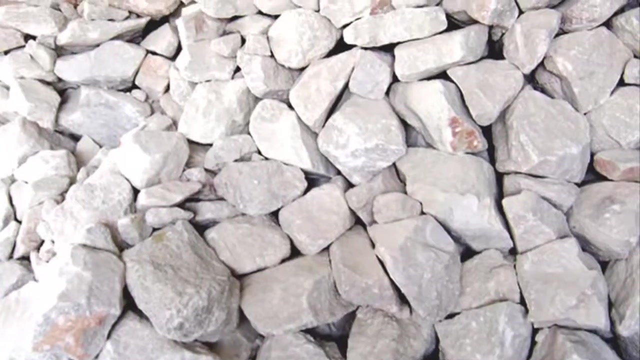 Much like trees, coral produce growth rings which vary based on oceanic conditions like ocean surface temperature, nutrient availability and water clarity. But this is where the similarities between trees and coral end. Rather than using wood, coral produce their growth rings out of calcium carbonate. 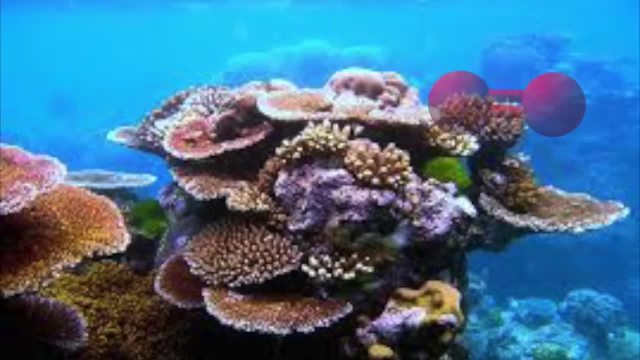 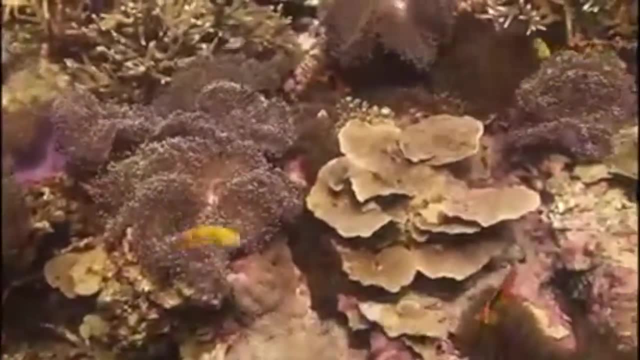 This gives the coral the ability to keep a record of the chemical composition of the water around it. This is a big deal, as this data can tell us a lot about various oceanic and therefore climatic conditions for every year that the coral has been growing. 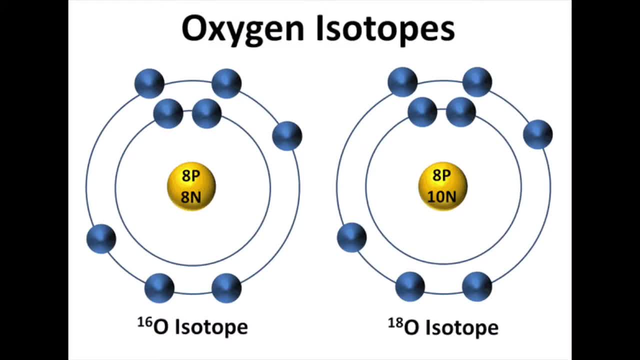 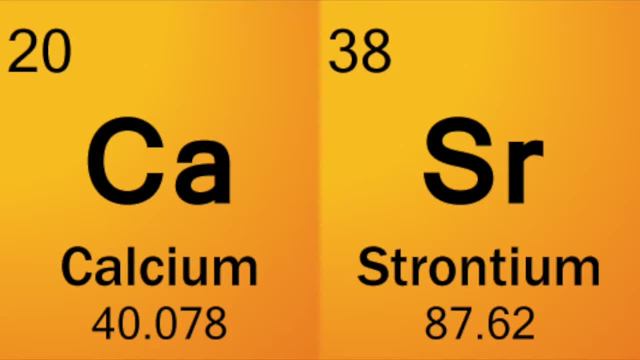 Firstly, climatologists can measure the ratio of light and heavy oxygen for each growth band, with more light oxygen indicating higher ocean temperatures and more rainfall. Secondly, measuring the ratio between calcium and strontium can indicate ocean temperature with a higher concentration of calcium. 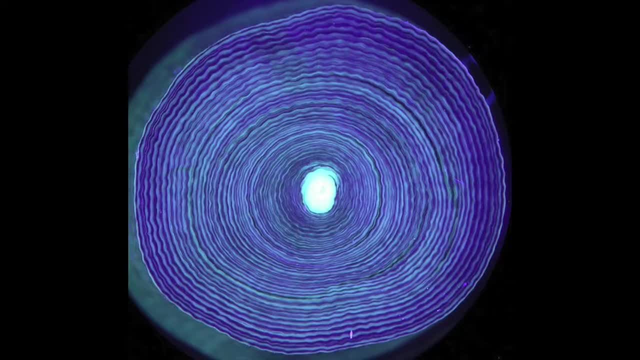 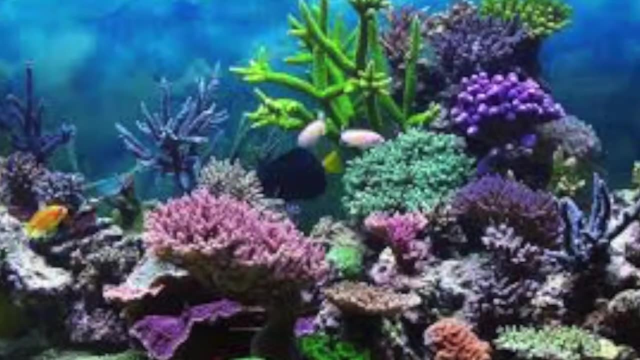 This is what every year looks like. Comparing these two ratios and the width of growth rings across multiple samples can give us a clear picture of what the climate was like in the area of the ocean where the sample was taken. But this leads us to a problem. 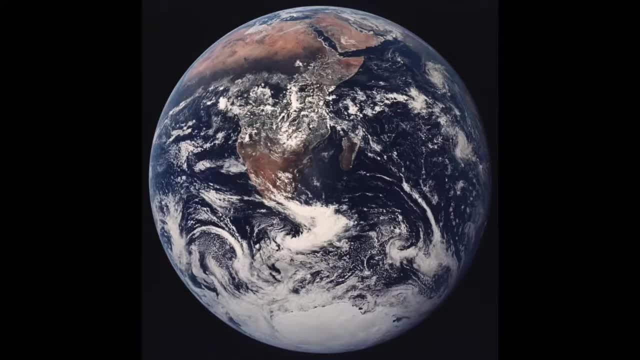 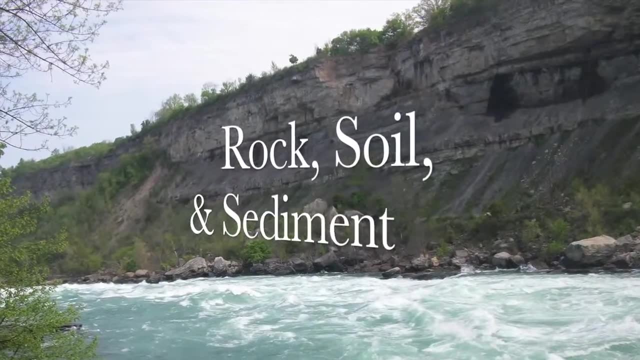 Coral reefs only grow in tropical regions of the ocean. so how do we find out what the past climate was like in other parts of the world? Conclusion, Conclusion, Conclusion, Conclusion. soil that you walk on every day contains volumes of evidence of our past climate, and the same 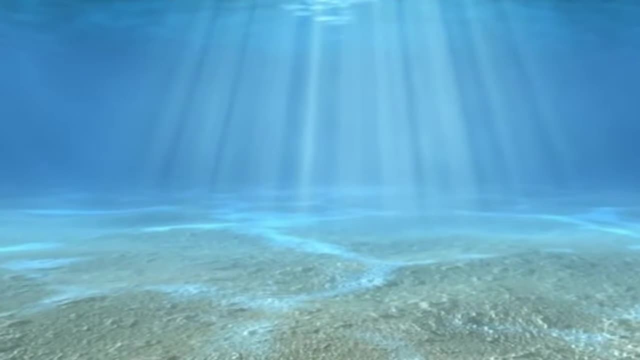 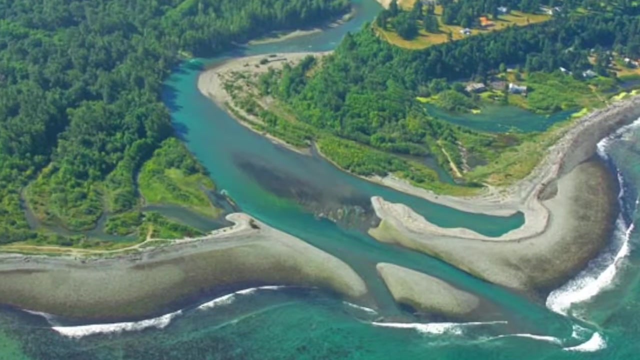 goes for the sediment beneath the ocean floor. At any given time, new layers of soil and sediment are being deposited on the land and the ocean floor at a very, very slow rate Over millions of years, due to heat from the center of the earth and pressure from layers. 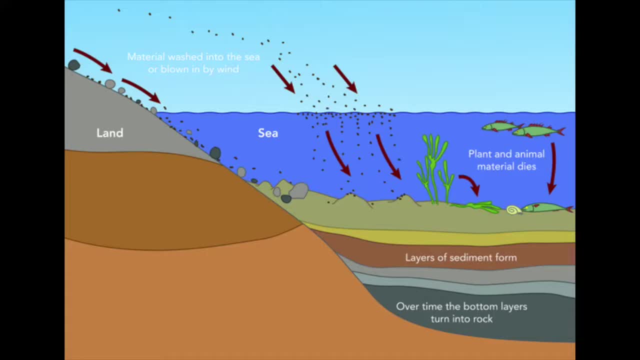 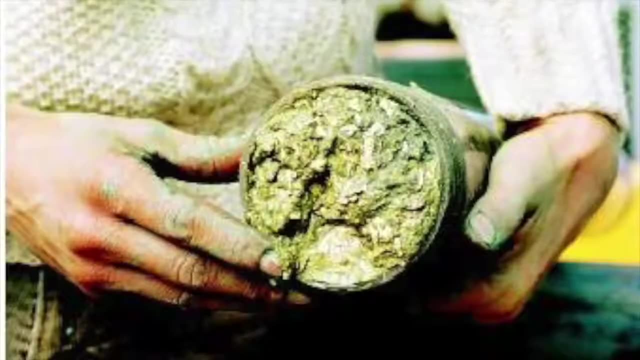 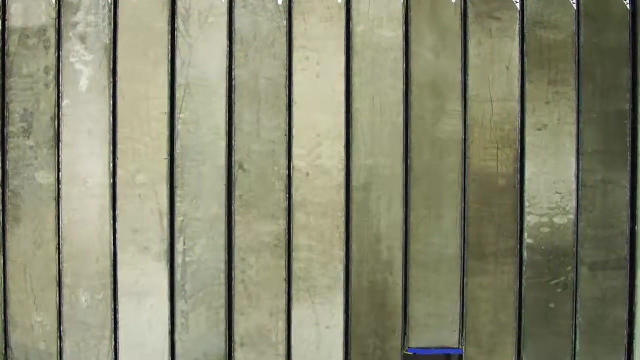 above these layers turn into rock, and any organisms that become trapped in the soil and sediment turn into fossils. Scientists excavate the soil and rock and take sediment cores from various areas of the land and ocean respectively. The samples are then dated using methods like radiometric age dating, though generally the deeper the fossil or rock. 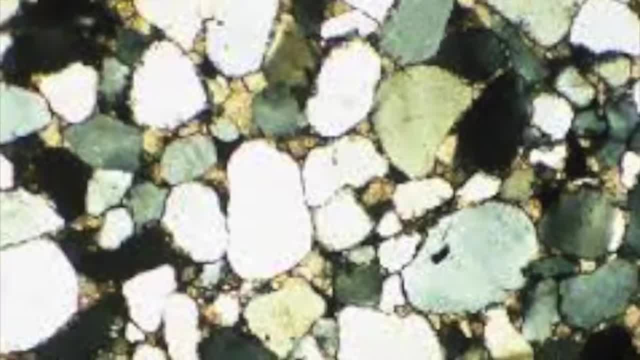 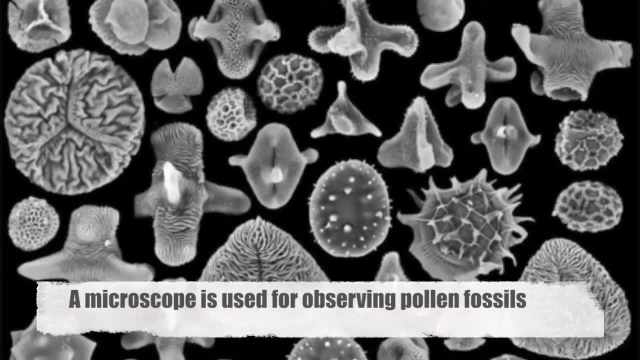 the older it is. The samples are then observed, sometimes under a microscope. Paleontologists observe what type of fossils are found, where and when, and paleologists do the same for pollen fossils. Paleontologists do the same for pollen fossils. This can help determine if its a frosted eggs. 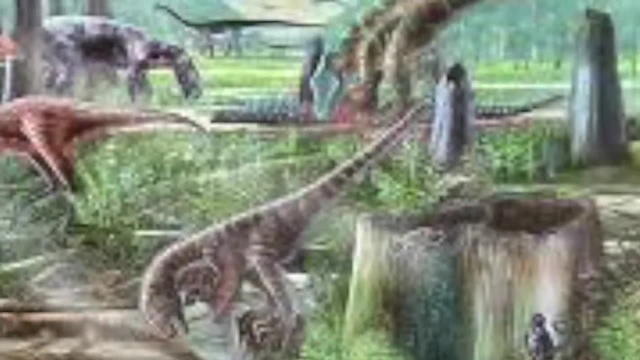 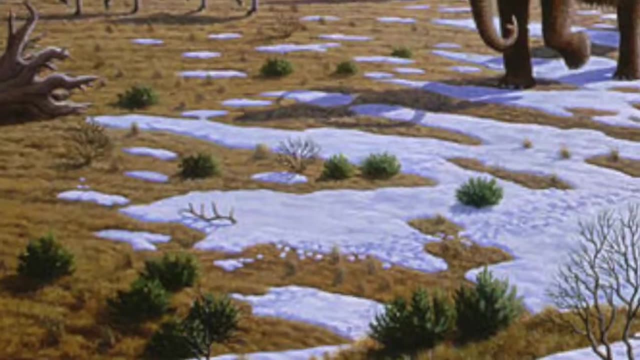 what organisms, and in the case of pollen, plants, lived where at what times, and by comparing that with what we already know about what types of climates these organisms preferred, we can gain a broad idea of what the climate must have been like at that time. But this is not the only thing rocks can tell us about our 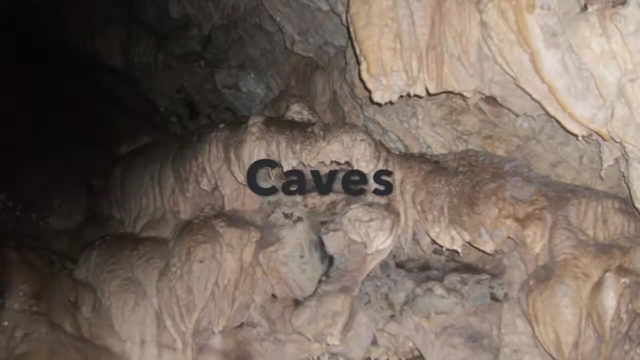 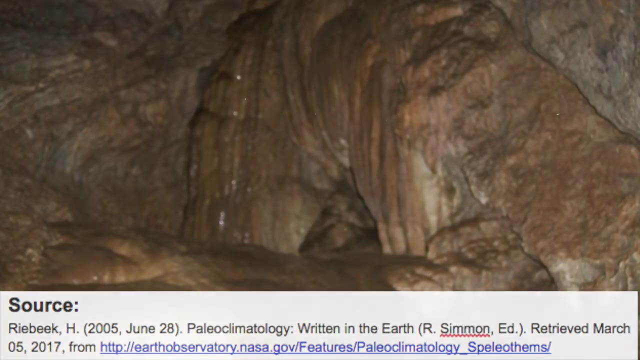 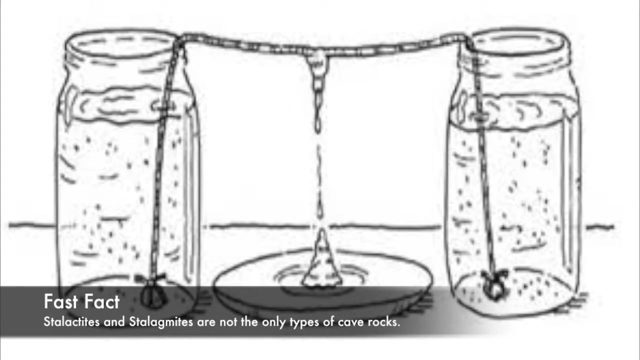 past climate. The rocks in caves can also be an indicator of the climatic conditions of an area. Stalactites and stalagmites, found on the roof and floor of caves respectively, form, as water deposits- minerals- onto these rock formations. These formations grow faster during times of wet rainy weather, as 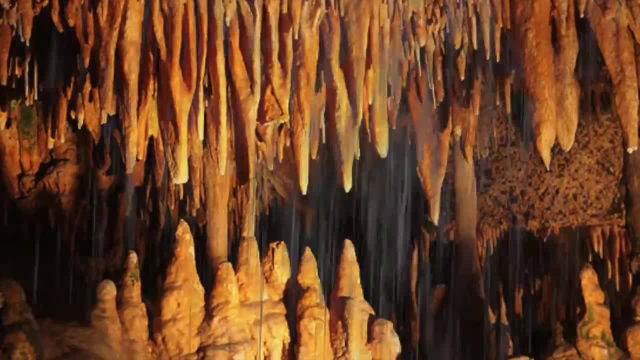 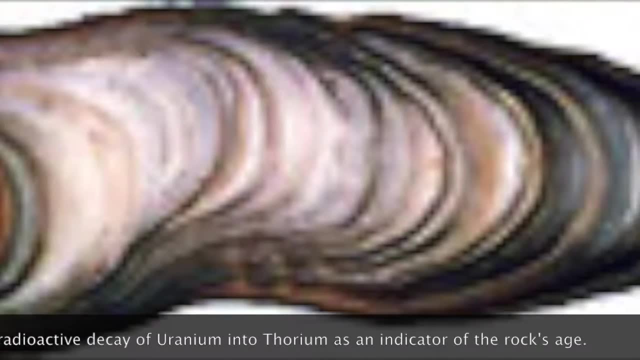 more minerals get deposited onto them by an increased amount of water. These rocks can then be dated using radiometric age dating to determine which years experienced more growth and, through that, how wet these years were. But this is not the only climate record that water. 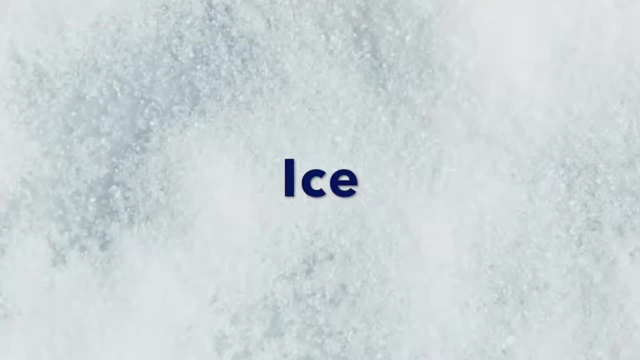 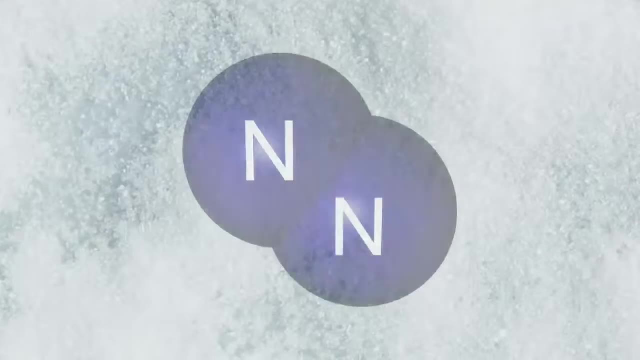 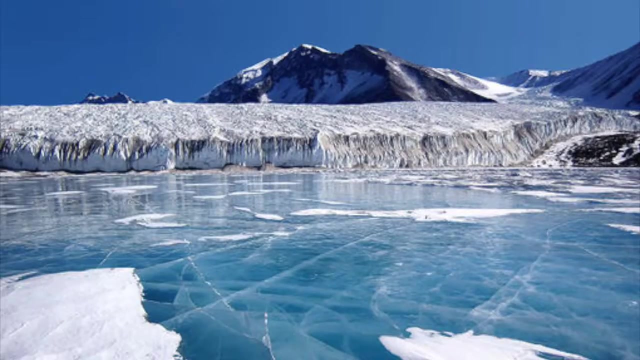 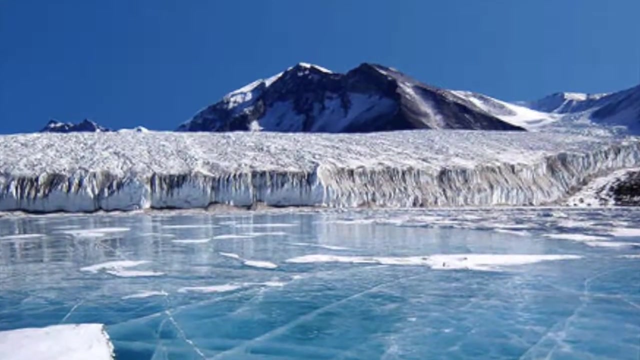 helps us keep. As ice forms, air bubbles are trapped inside. These air bubbles contain the concentration of gases that were present in the Earth's atmosphere at the exact moment at which they were trapped. In areas like Antarctica and Greenland, where some of the ice hasn't unfrozen for millennia, this provides a record of 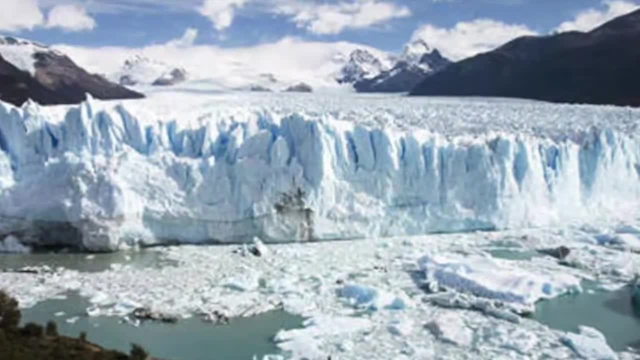 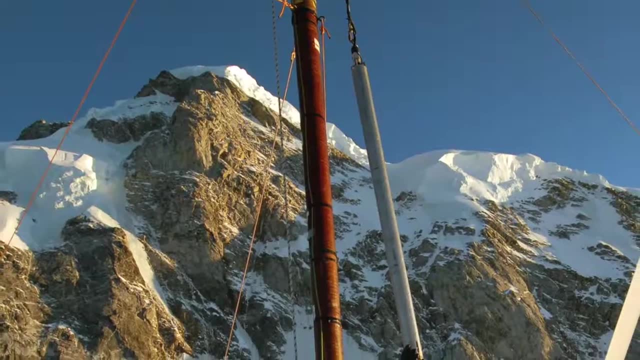 the concentration of different gases in our atmosphere, dating back 100 to 123,000 years in Greenland and over 800,000 years in Antarctica. Scientists can observe this record by taking and analyzing ice cores from these areas, once again using the basic. 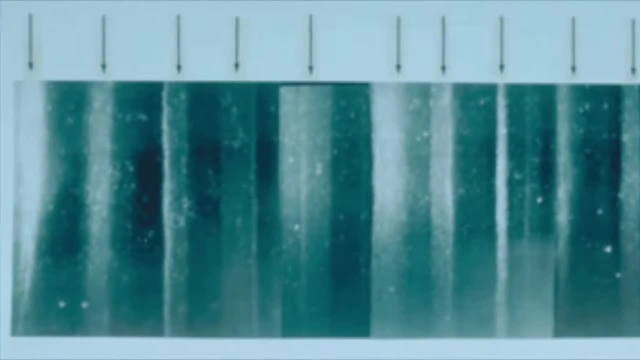 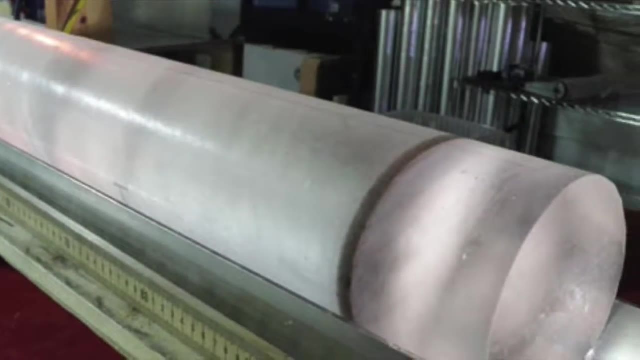 principle: the further you go down, the older it is. These samples can be more accurately dated using various events like major volcanic eruptions as indicators. During these events, concentrations of certain gases like sulfur dioxide are known to have been the cause of the. 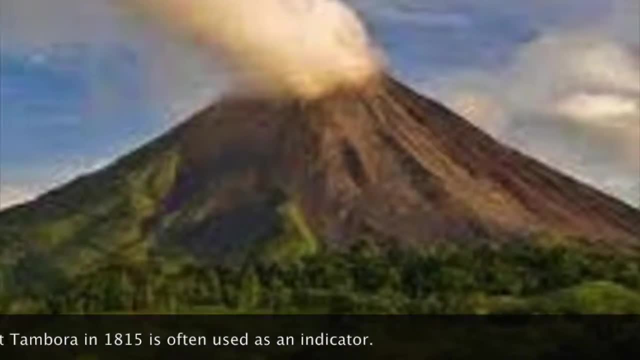 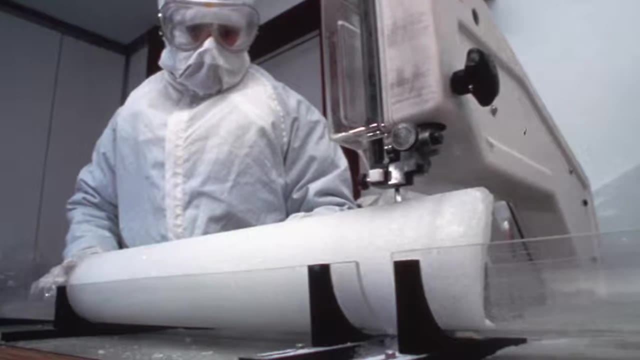 rise in air temperature, and the rate of the rise in air temperature has been significantly higher, And observing that in a layer of ice can tell you when that layer was formed and when the areas around it were formed. The ice cores are sliced into thin slices. 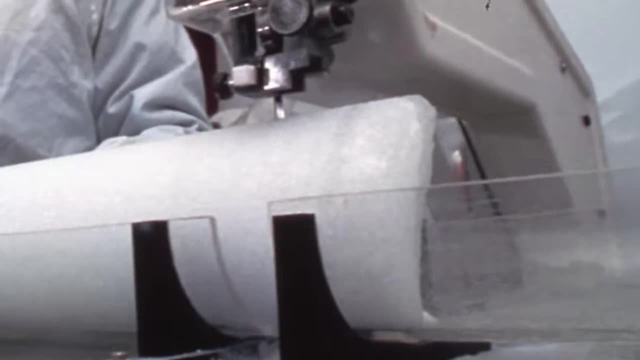 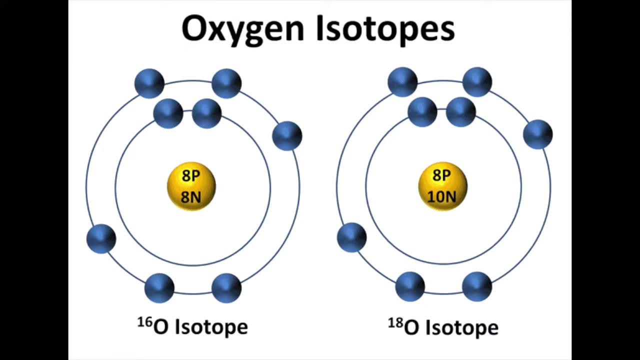 like meat is at a deli, and these slices are tested for various gases. Oxygen is one of the gases tested for, as the ratio of light to heavy oxygen atoms indicates what temperature the air was when the air bubble was trapped. The more light oxygen there is, the cooler. 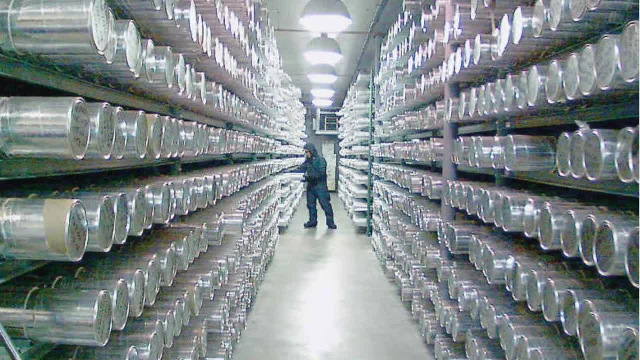 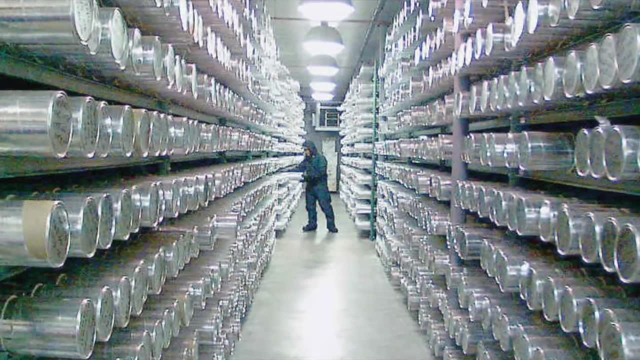 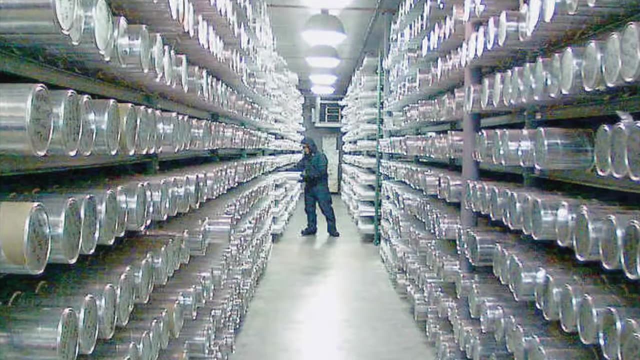 it was. As an added bonus, this ratio can be used to more accurately date the sample, As annual fluctuations in temperature change this ratio. so every year there will be a high point and a low point in the level of light oxygen. The samples are also tested. 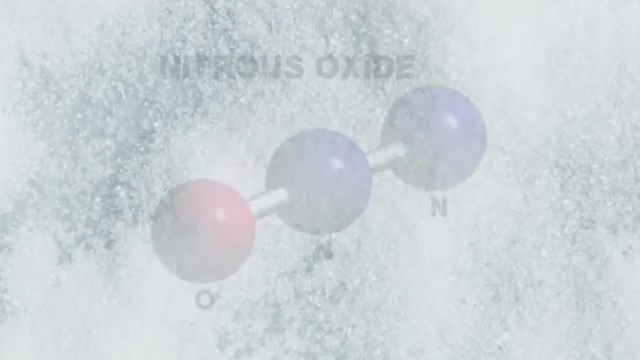 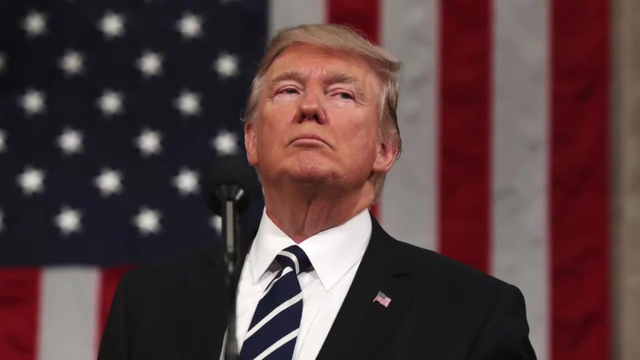 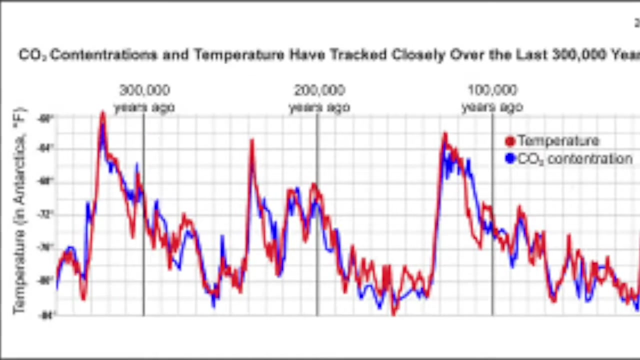 for various greenhouse gases like carbon dioxide, nitrous oxide and methane, as higher levels of these gases indicate higher temperatures. Broom, We do not know that these gases indicate higher temperatures? Ah, yes, we do By comparing the temperatures indicated by the ratio of light to heavy oxygen. 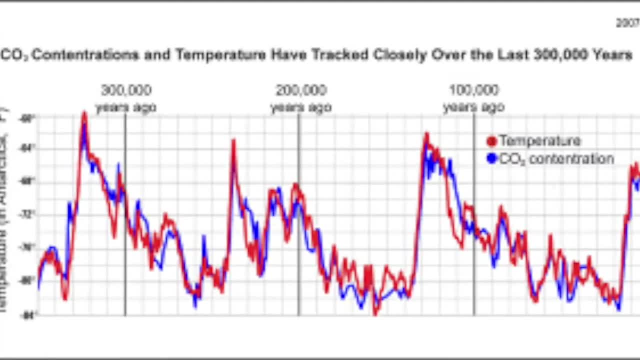 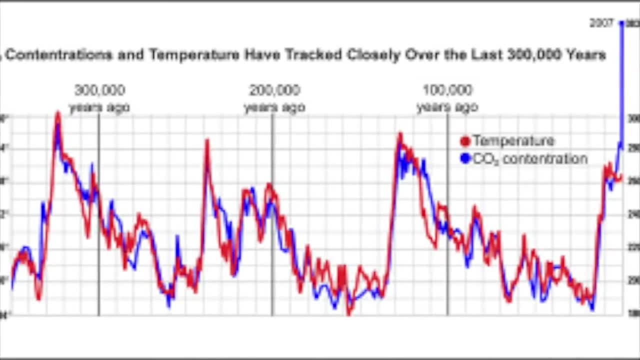 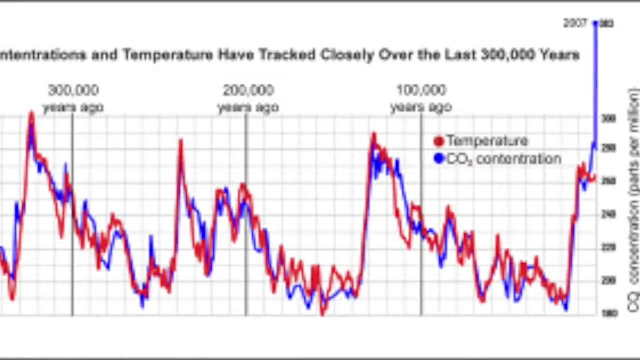 atoms to the levels of these greenhouse gases found in the same air bubbles, and by comparing the data from the ice cores to data from other proxy records and direct records, climatologists have concluded that there is a correlation between higher temperatures and higher levels of these greenhouse gases, and therefore higher levels of greenhouse gases are linked. 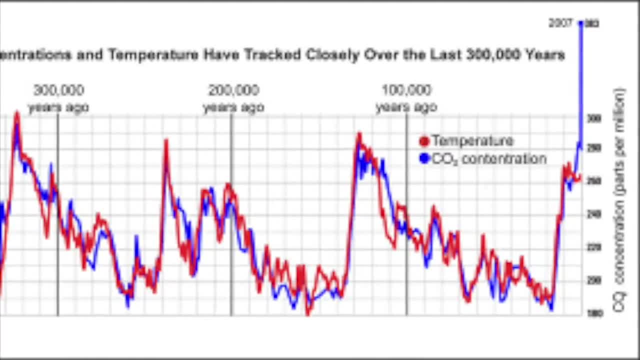 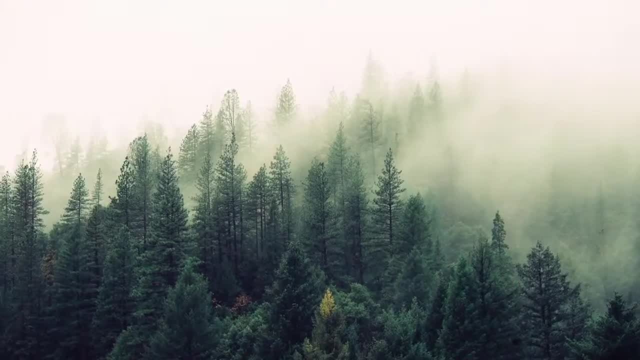 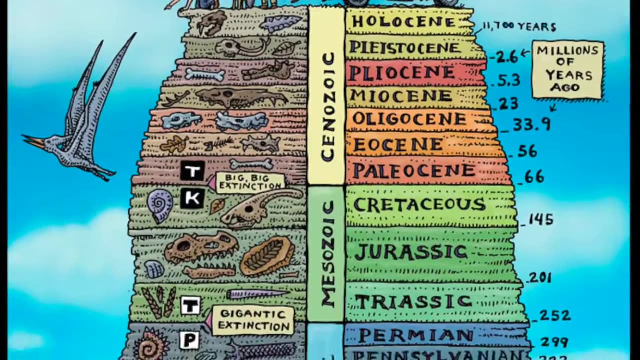 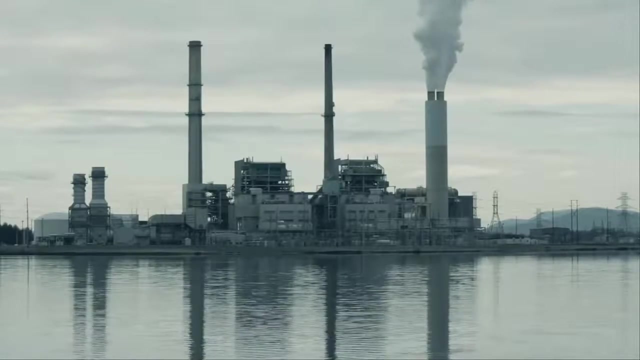 to higher temperatures. This is why proxy records are so important when it comes to proving climate change is real. We only started recording climate records very, very recently. in both geologic and human history, CO2 levels were not consistently recorded until the 1950s. Proxy records provide: